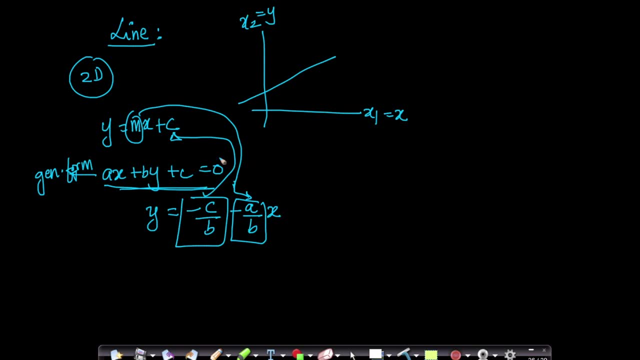 to interpret, and this is much more general. If my axes are x1 and x2, I can rewrite this equation as a: times x1 plus b, times x2 plus c equals to 0.. Instead of using abc, let me use a different notation, because if you want to do it in 10 dimensions, how would you write it? 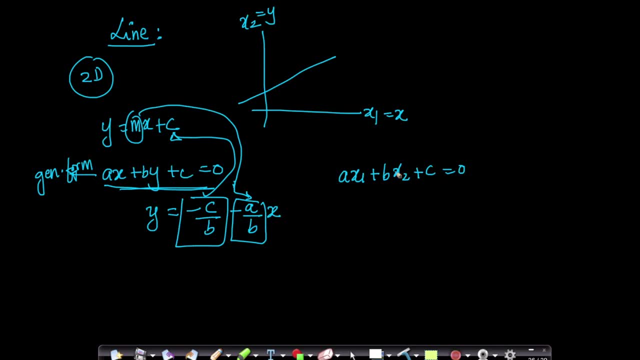 I will have to use all the alphabets If you want to use 100 dimensions. I do not have enough alphabets. I can write as: w1, x1 plus w2, x2 plus w0 equals to 0.. Instead of a, I am writing w1.. Instead of b, I am writing w2.. Instead of c: 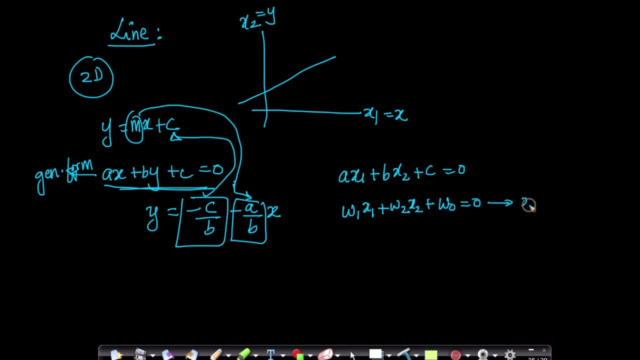 I am writing w0.. This is the equation of a line in 2D. What about 3D? Some of you might have learned 3D coordinate geometry in undergrad. For those of you who do not recall it, if I have my axes as x1,, x2, and x3,, the equivalent. 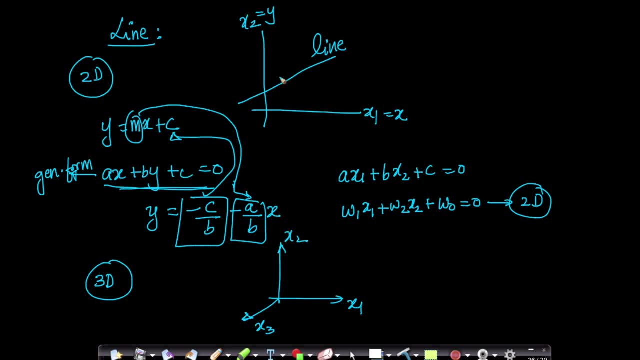 of a line is a linear surface in 2D. The equivalent idea of a line in 3D is a plane. The equation of a plane, for those of you who might remember it, looks like this: ax plus by, plus cz plus d equals to 0.. This is an equation that some of 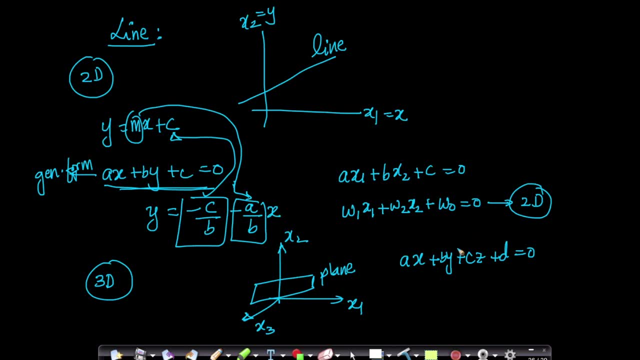 you may be familiar with because you took a math course in your undergrad first year and second year. Let us just generalize it. What this looks like is w1, x1 plus w2, x2 plus w3, x3 plus w0 equals to 0.. This is the equation of a linear surface. This is the equation of a plane. 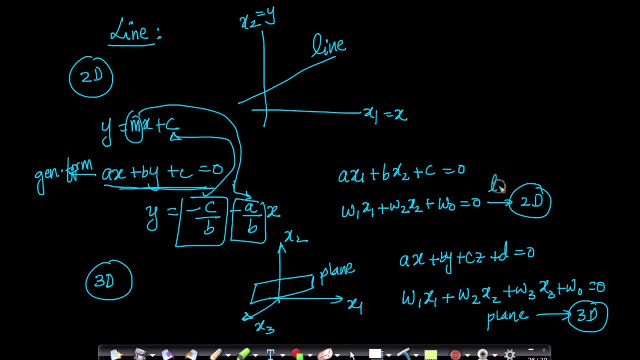 This is a plane, This is a line. The idea, the equivalent idea of a line in 2D is plane. So line in 2D is nothing but plane in 3D. Now the immediate question is: what about? 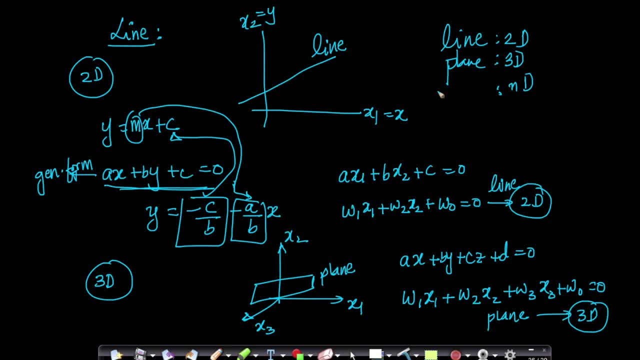 n-dimensional space. What is it called? It is called something called a hyperplane. Hyperplane is basically a generalization of the concept of a line or a plane to higher dimensional space, Because, if you think, line is called a linear surface because it 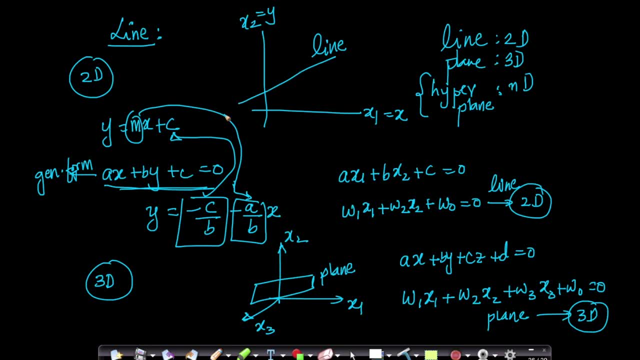 separates your whole region with a simple linear structure like a line or a plane, into two regions: One region on one side of the line, the other region on the other side of the line. Similarly, a plane can separate your 3D surface, your 3D volume into two regions. 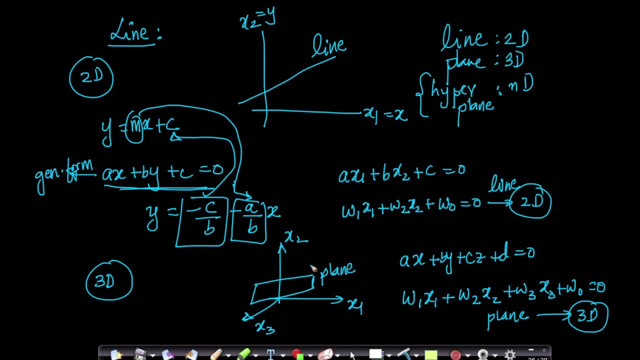 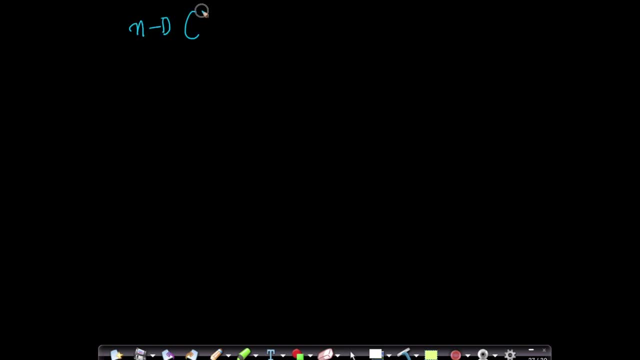 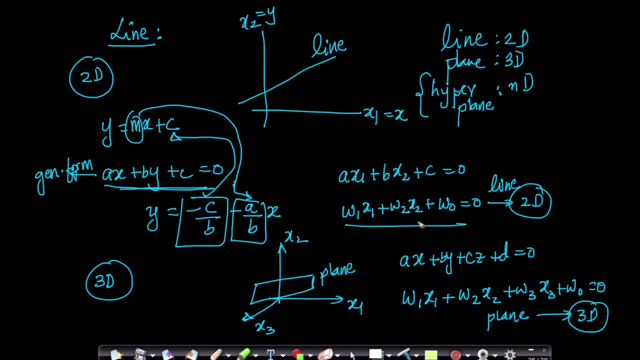 one above the plane and one below the plane. So the immediate question is: what is the equation of a plane in n dimensions? Suppose, if I have n dimensions, what is the equation of a hyperplane? You could have easily understood that by just looking at the form of this. This is 2D. 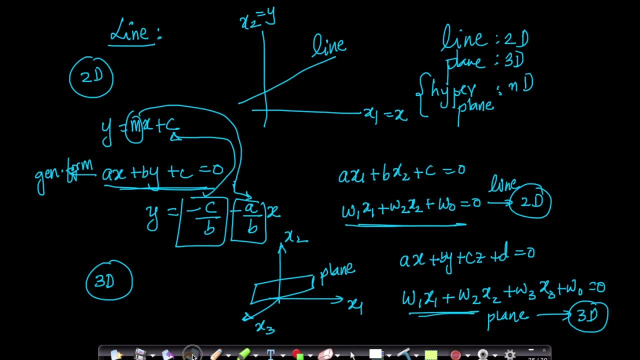 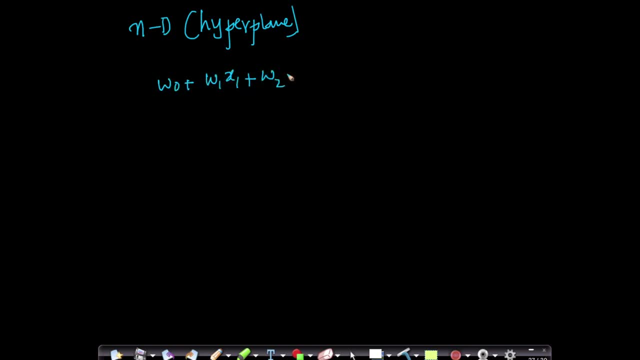 This is 3D. Now just let us extend it and see what will it be in nd. In nd, it will be w0 plus w1x1 plus w2x2, so on, so forth. Since we have n dimensions, wnxn equals to 0.. This is the 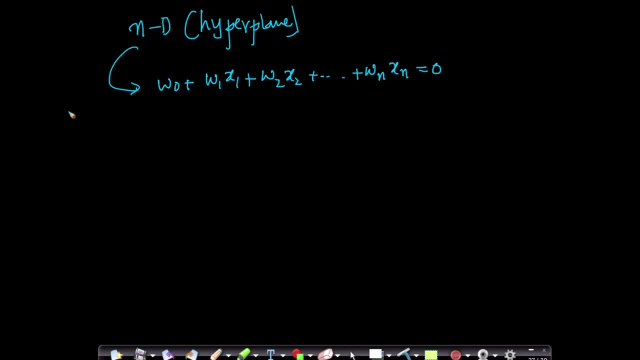 equation of an n-dimensional plane. So this is the equation of an n-dimensional plane. Now the immediate question we get is: this is too cumbersome to write. Is there a more concise way of doing it? Of course there is. We can use summation here. Summation i: 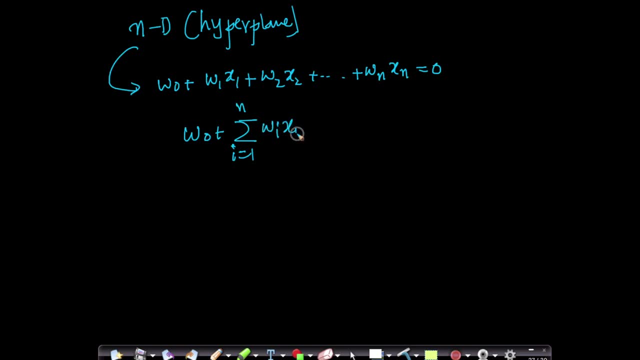 equals to 1 to m. wi xi equals to 0.. Now is there a better way to write this still further? This is still good. This is certainly much more concise way of writing the equation of a hyperplane in n-dimensional space than writing out this whole expression, So let 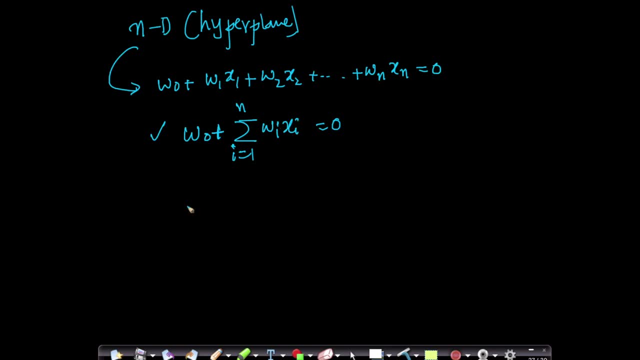 us continue. There is a slightly more interesting way of doing it, which is I can write it as w0 plus. imagine if I create a vector right w This vector, I will call it w. So those of you who remember how to multiply two vectors or multiply matrices, you will. 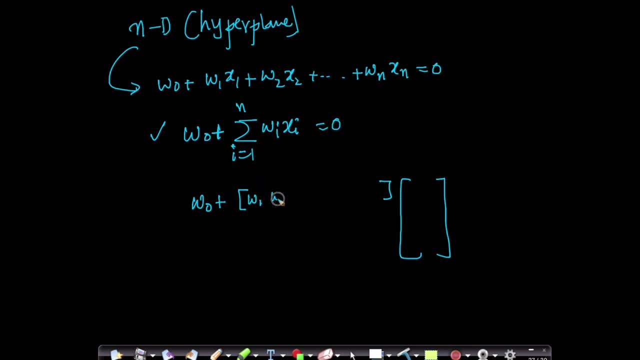 quickly recognize this. Let us assume I have w1, w2, so on, so forth. wn here. Imagine if I have w1, w2, so on, so forth. xn here. This is nothing but a vector notation. This is: 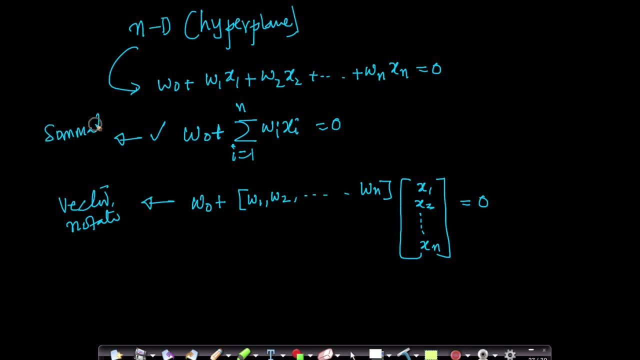 nothing but a summation notation. right, I am not changing any formula here, I am just changing the notation slightly. So what does this product look like? So, when you multiply this vector with this vector, those of you who have studied basic matrices and matrix, multiplication, probably in your 11th grade or 12th grade, you will be able to see that this is a vector. So when you multiply this vector with this vector- those of you who have studied basic matrices and matrix multiplication- probably in your 11th grade- you will easily. 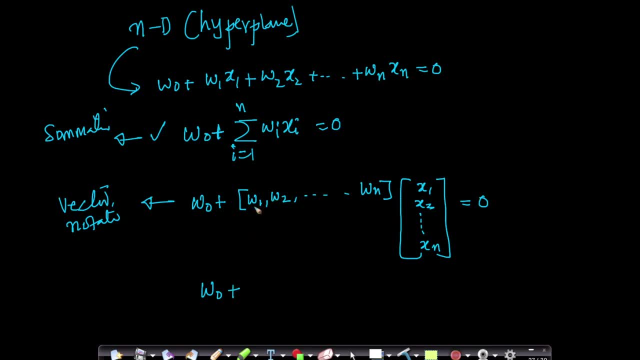 recognize this. So this is nothing but w0, plus the first component here gets multiplied with the first component here, right, which is nothing but w1, x1.. And then you add: take the second component, multiply it with the second component, which is w2, x2, and so 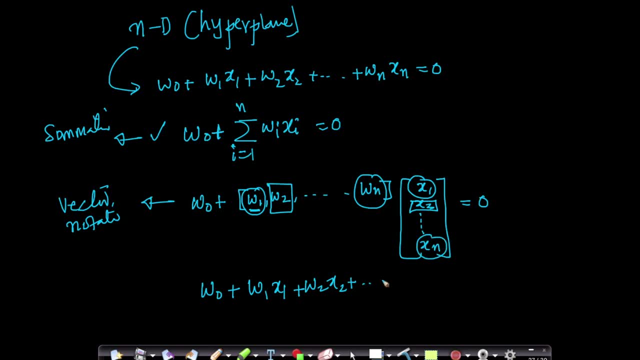 on so forth. Take your last component, multiply it with the last component, which is wn. xn equals to 0. So this is a vector notation of writing it And we will use this notation a lot. Immediately after this section, we will understand what is a dot product and we will write this: 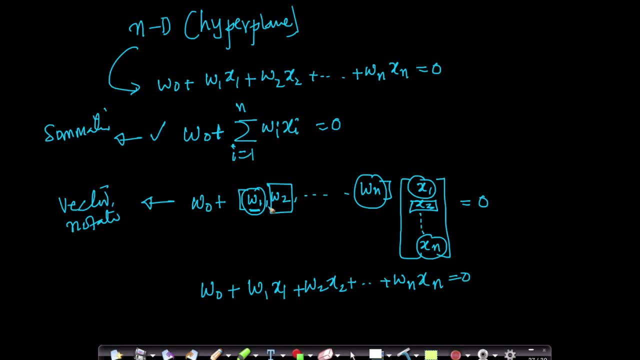 in a much more concise form using vector notation. Now, this vector, I can, since this vector, I can think of this as a vector w. I can think of this as a vector x. right, This vector x has n rows. right, it has n rows and it has only one column. This vector w has one. 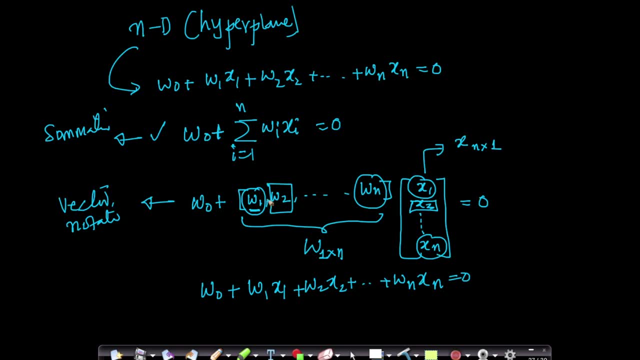 row and it has n columns, right? So if you recall the vector, the matrix multiplication, so you can multiply 1 x n with n x 1 to get a 1 x 1 matrix. So, those of you who remember, 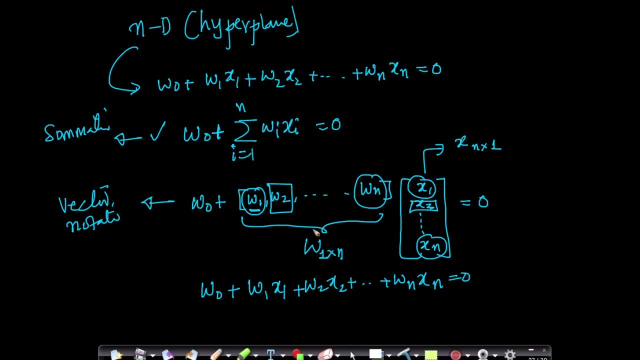 simple matrix multiplication will quickly understand that what we have here is nothing but a simple matrix multiplication of a row vector with a column vector, right. So this is. this is how we represent a plane. We look at a plane, or hyperplane, in n dimensional. 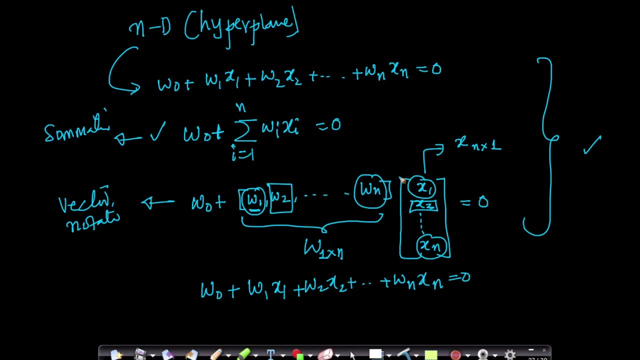 space. We look at many properties of lines and planes in the next few videos. 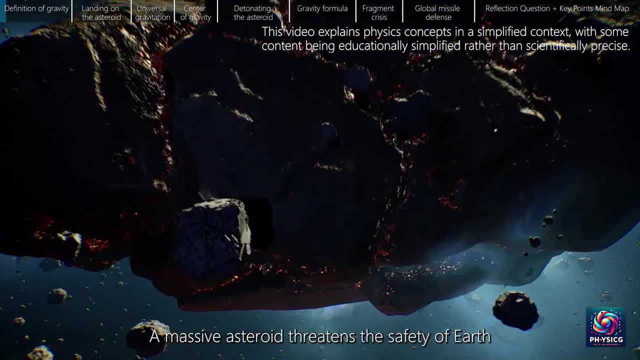 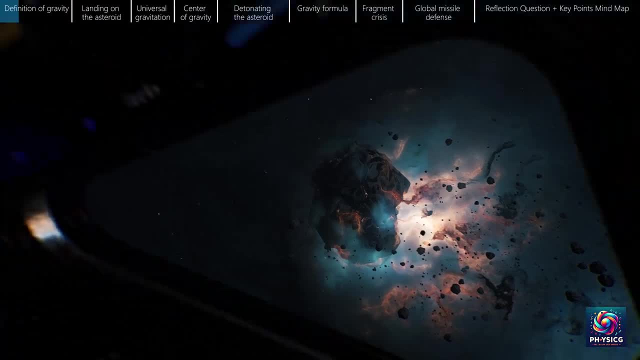 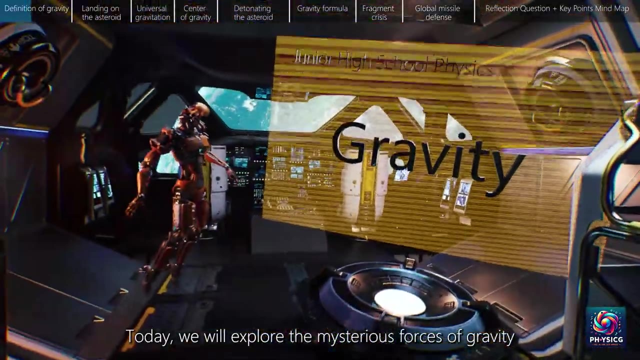 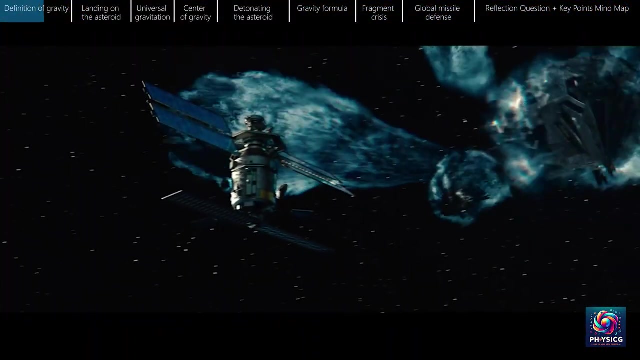 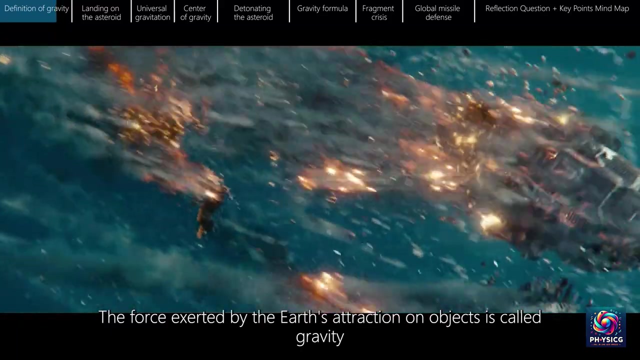 We are facing an unprecedented crisis. A massive asteroid threatens the safety of Earth. We must take action. Welcome students to this lesson on gravity. Today we will explore the mysterious forces of gravity, Understanding how it affects our world and the entire universe. Did you see that thrilling scene? The force exerted by the Earth's attraction on objects.